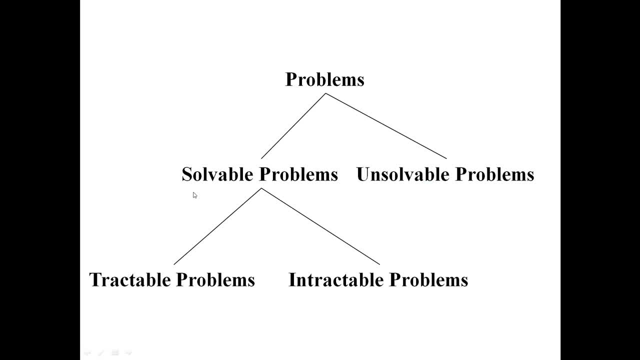 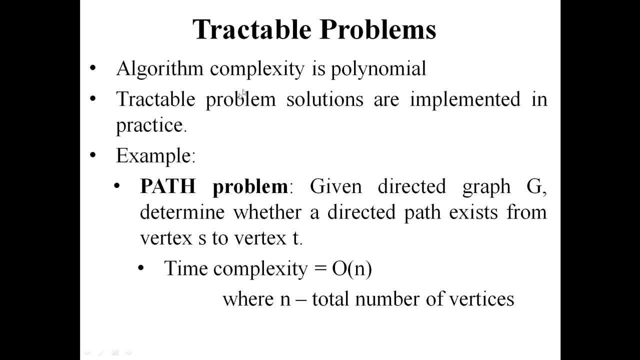 Solvable problems can be again divided into tractable problems and interactable problem Here the first one is tractable problem. Problem solve: chayyan attikunna, complexity, polynomial time, anankil. it is called tractable problem. Tractable problem solutions are implemented in. 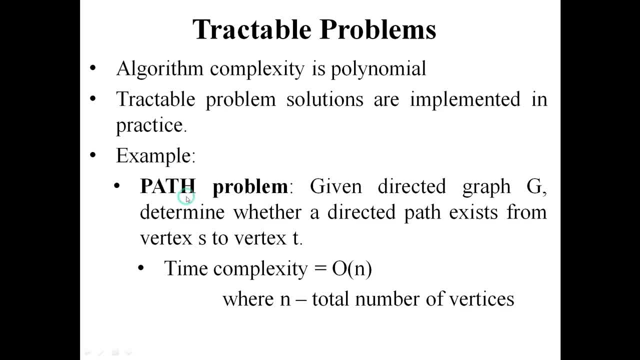 practice. Example is path problem. This is a directed graph. There are two vertexes, S and T. The path problem is whether a path exists or not. The complexity of this algorithm is big. I of n, where n is the total number of vertices. 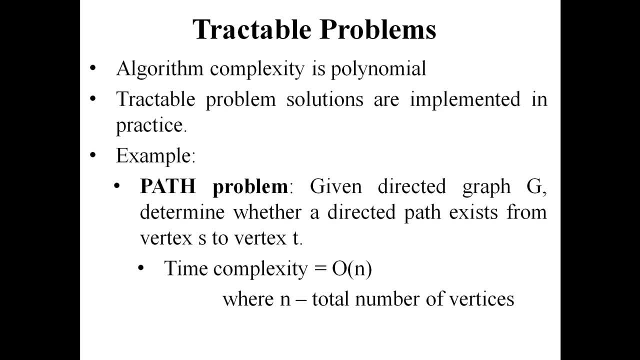 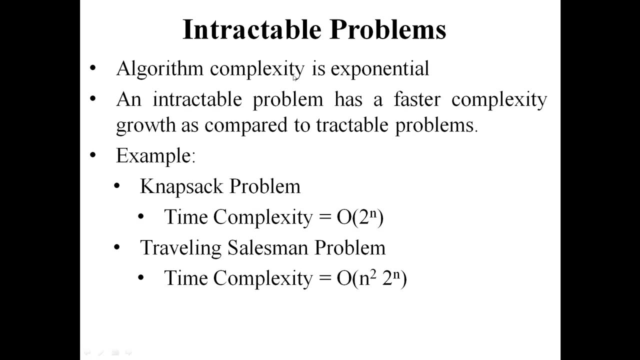 Algorithm complexity: big I of n n. square n cube is a polynomial time complex. Here the complexity is big I of n. This is a polynomial time complex. Path problem is a tractable problem. Second one is interactable problems: Algorithm complexity, exponential time. It is called the interactable problem. 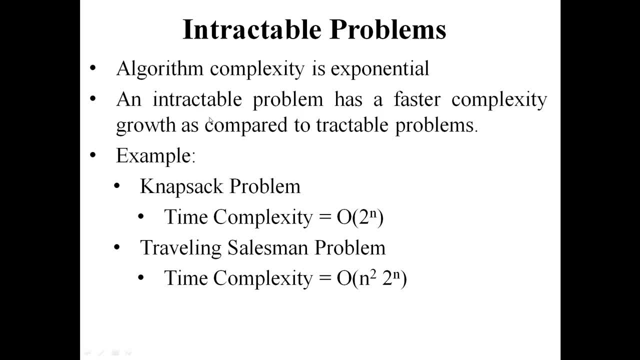 An interactable problem has a faster complexity growth as compared to tractable problems. knapsack problem: its complexity is big guy of 2 raised to n. travel in salesman problem: complexity is equal to big guy of n. square into 2 raised to n isn't the lm complexity. 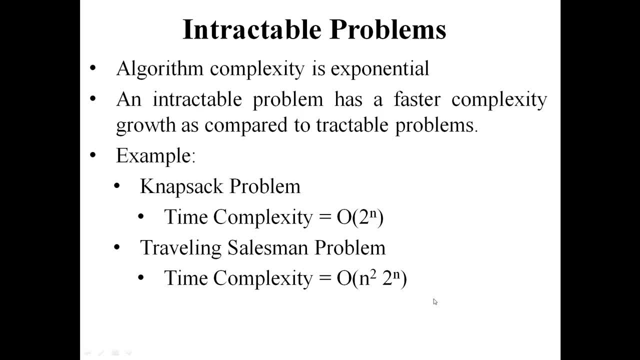 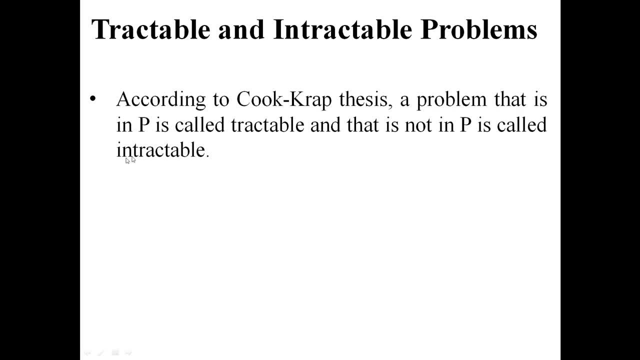 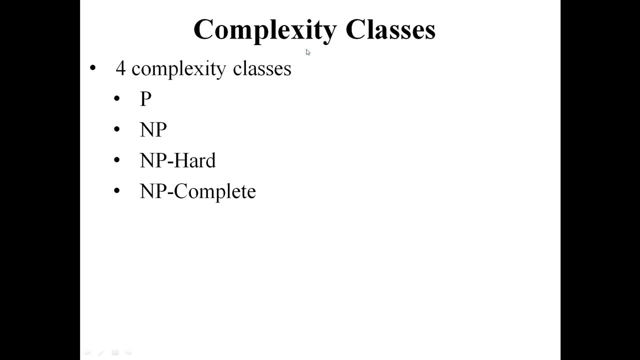 exponential time on. so these all are belongs to intractable problem. according to coop crop, this is a problem that is in p is called tractable and that is not in p is called intractable. complexity classes. there are four main complexity classes: p, nb, nb hard and nb- complete. 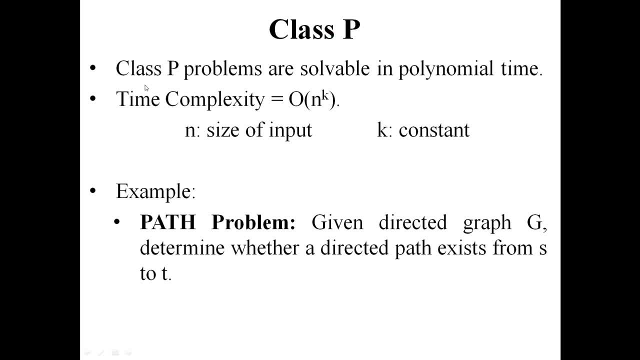 first one is class p. class p problems are solvable in polynomial type. its complexity is equal to big guy of n raised to k. here n is the size of input and k is a constant big guy of n, power, k, nb. These are the problems of algorithmic complexity in class P. 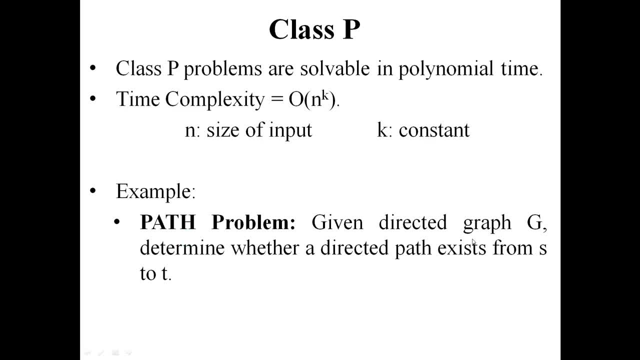 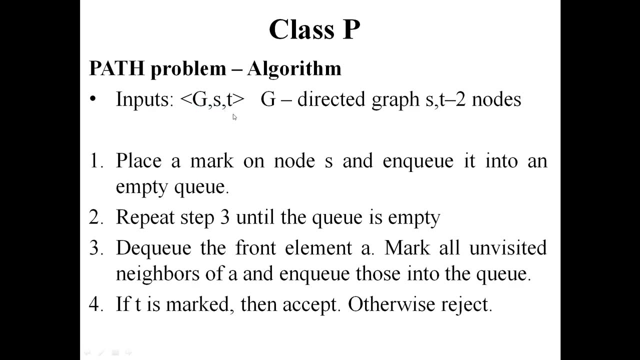 Example: path problem. Given directed graph has two vertices: S and T. Does S to T have a path? That is path problem. Its algorithm is this: Inputs are G, S and T. G is the given graph and S and T are the two vertices. 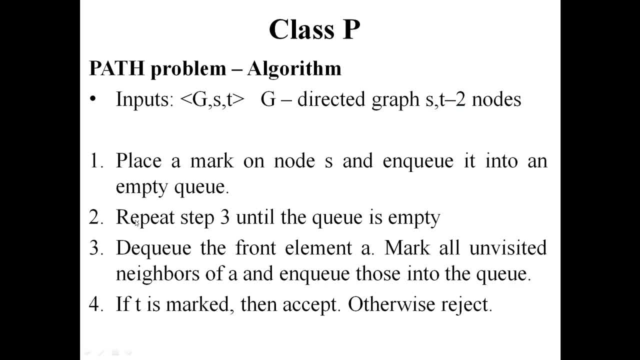 Algorithm. Initially all nodes are set as unvisited. Then take the node S, mark it and enqueue it to an empty queue. Step number 213 is a loop. Delete a node from the queue, Then enqueue all its unvisited neighbors to the queue. 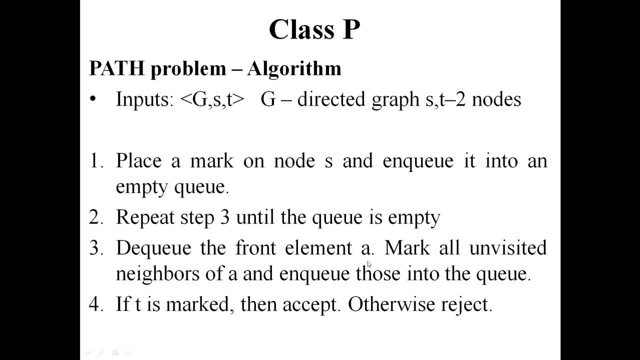 Again one element from the queue, Then dequeue. All the unvisited neighbors of that node are visited and enqueued to the queue. This process continues In the situation where the queue is empty. exit from this loop and come to step number 4.. 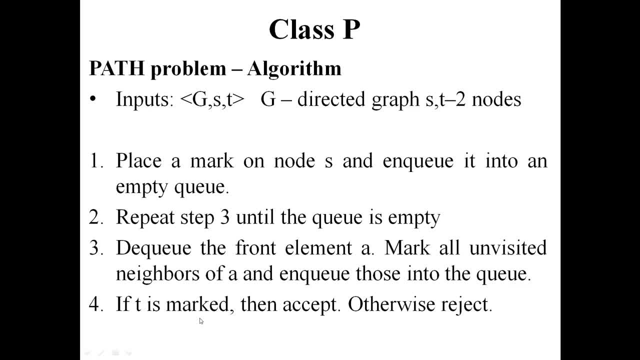 Check if T is visited. If it is visited, S to T has an exit, So accept it, Otherwise reject it. Then find the complexity of this algorithm. Step number 1 and 4 are the constant complexity. 2 and 3 are a loop. 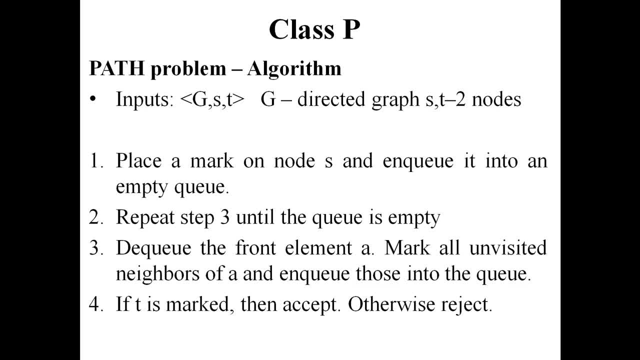 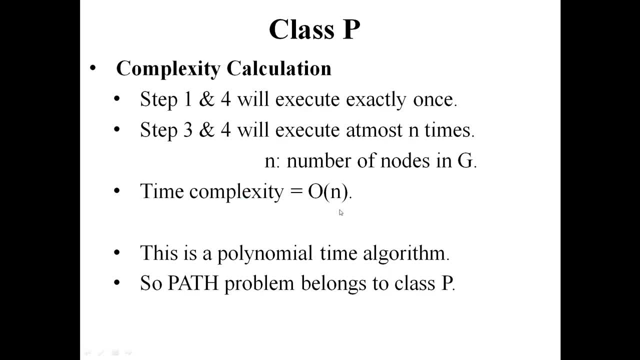 This loop is at most n time. I treat you. Where n is the number of nodes in the graph, So the time complexity is equal to big guy of n. So this algorithm is a polynomial time algorithm. So path problem belongs to class P. 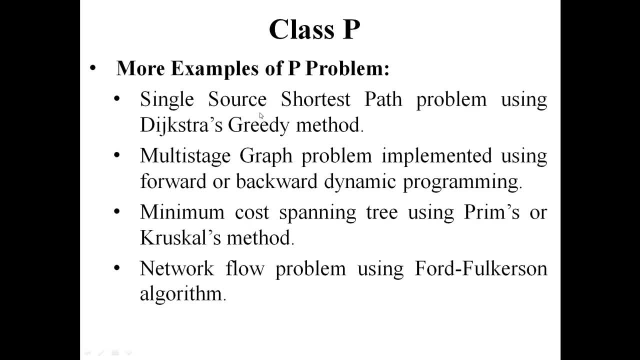 Few more examples: Single-source shortest path problem using Digextas Grede method, Multi-stage graph problem implemented using dynamic programming, Minimum-course span entry using Prem's or Kerkel's method, Network flow problem using 4-Furcursive algorithm, etc. 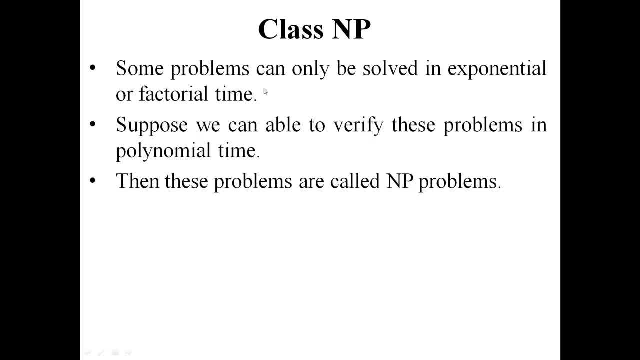 Class Nb. Few problems are not existing in the algorithm that solves them in polynomial time. Some problems don't exist in the algorithm that solves them in polynomial time. buttons simply don't exist in the algorithm. It can't be solved at polynomial time. 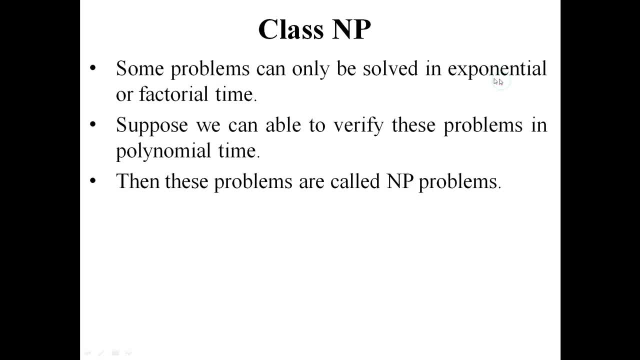 � Problems like this can be solved in exponential or factorial time. If such a problem can be verified in polynomial time, it is called NP problem. NP problem does not have a solution in polynomial time, but it can be verified in polynomial time. Example is Hamiltonian path problem. 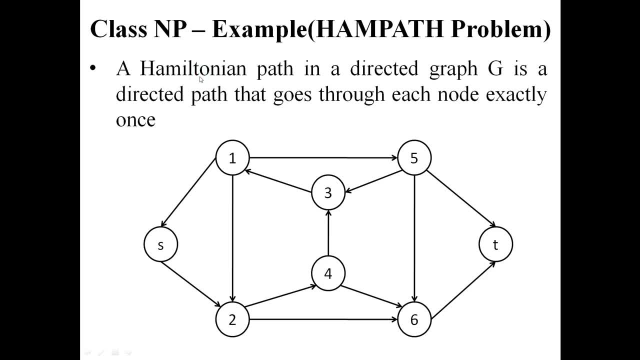 First of all, what is Hamiltonian path In a directed graph? if the path between two vertexes is covered exactly once, it is called Hamiltonian path. The Hamiltonian path in this graph is shown in red colour: Yes, 2,, 4,, 3, 1,, 5,, 6, 3.. 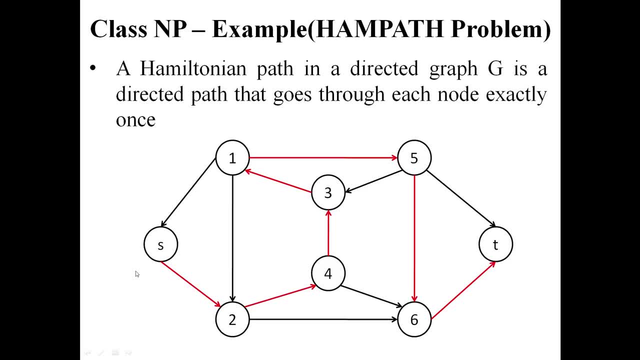 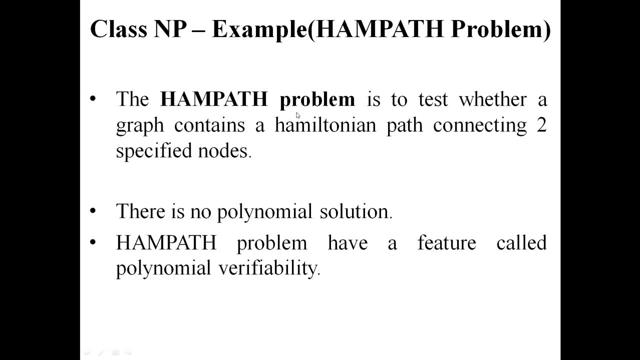 All the nodes are covered exactly once and reached T from S Hamiltonian path problem is whether a Hamiltonian path exists in a given graph or not. The Hamiltonian path problem is to test whether a graph contains a Hamiltonian path connecting two specified nodes. 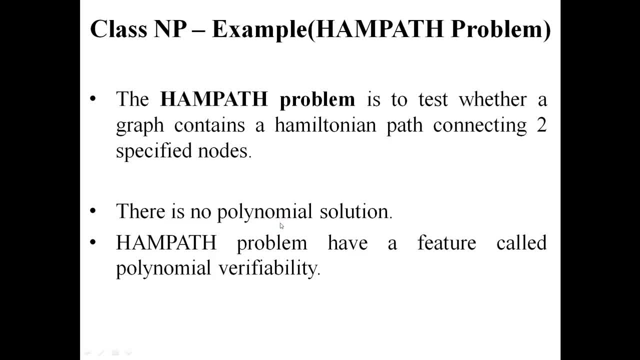 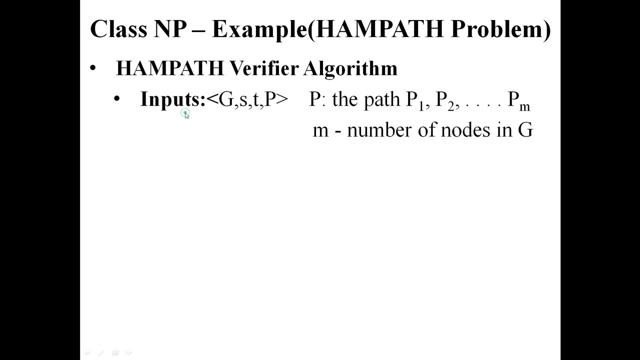 This problem does not have a solution in polynomial time, But there is an algorithm to verify this in polynomial time. Now we are going to see the verifier algorithm of Hamiltonian path problem. Inputs are G, S, T and P. G is the given graph. 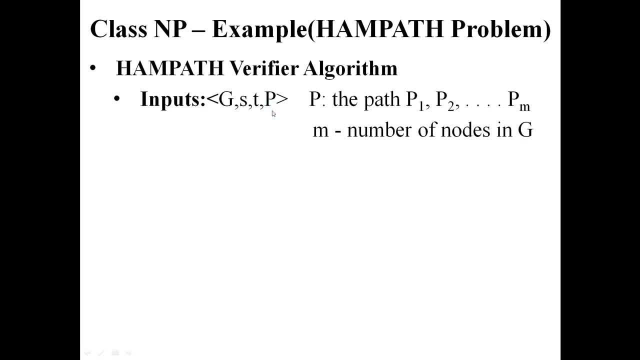 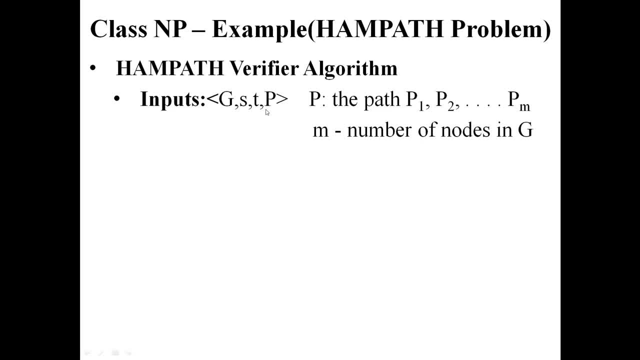 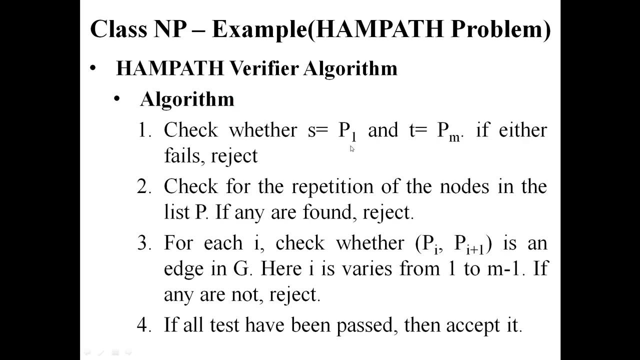 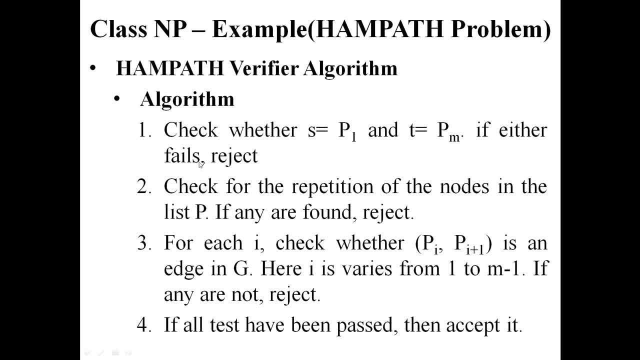 Is the Hamiltonian path from G to T, from S or P situation? just reject it. If first three cases are successful, we can say that, given graph G, Hamiltonian path is P. This is Hamiltonian path verifier algorithm. This algorithm complexity. 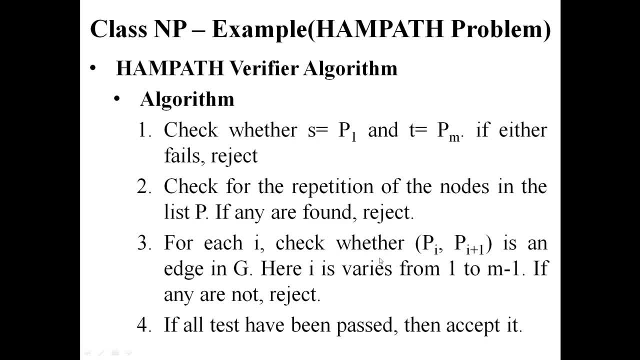 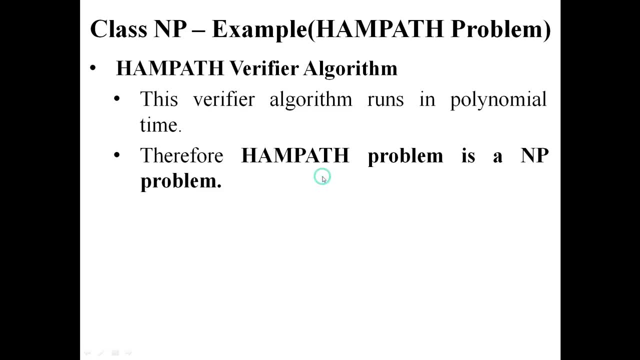 is in polynomial time. To find out if Hamiltonian path exists, we need a polynomial time algorithm. This algorithm does not exist. Verification exists in polynomial time algorithm, So we can say that Hamiltonian path problem is a NB problem. Another example is click problem. 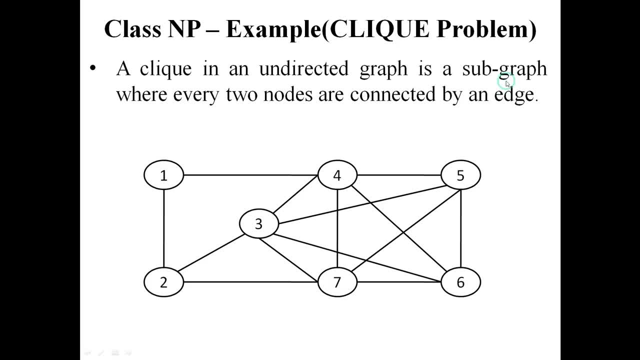 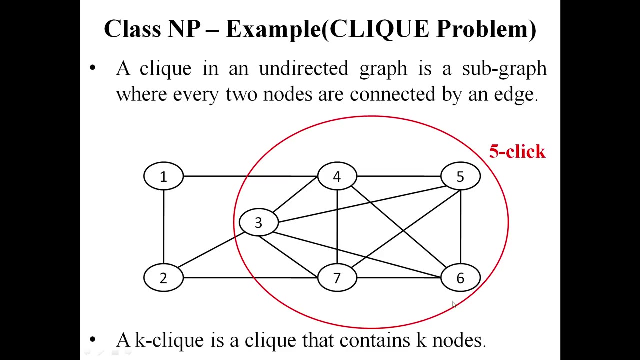 A click in an un-directed graph is a subgraph where every two nodes are connected by an edge. This is the given graph. If we say click in this graph, it is a click. This is a click with five nodes. If we say property, this subgraph is completely connected. 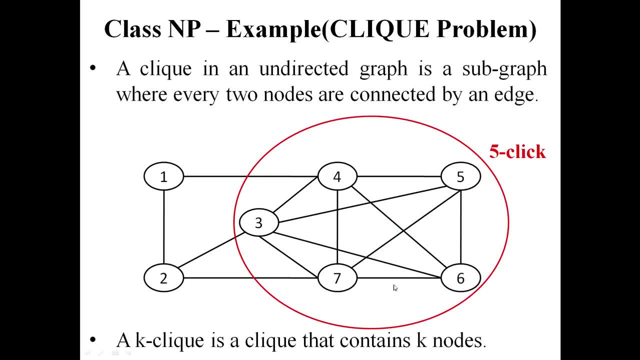 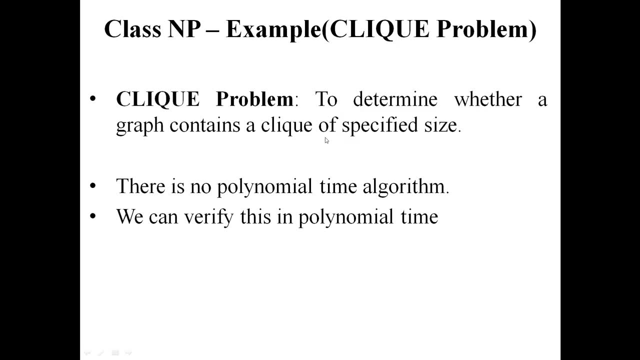 That means all the nodes have edges in between. A K click is a click that contains K nodes. This is a five click Click problem to determine whether a graph contains a click of specified size. This click problem is whether a click of finished graph contains a click of specified 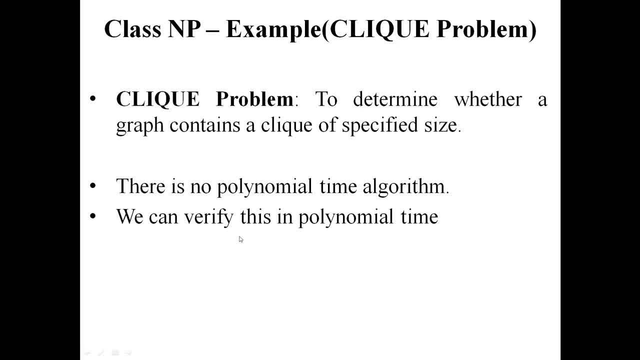 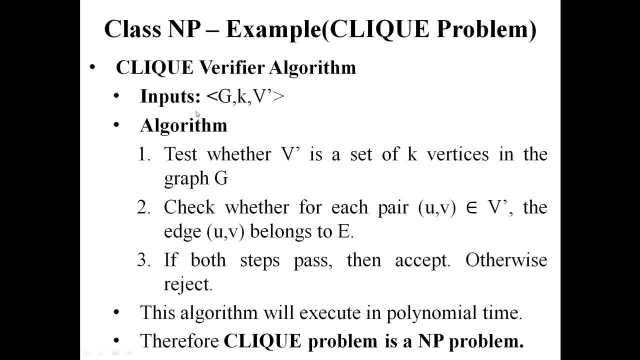 size. To solve this problem, there is no polynomial algorithm existing yet, But there is a bottom branch of polynomial time verification algorithm. This is that algorithm Inputs are G, K and V dash. G is the given graph and K is the rise of click. V dash indicates the distance. 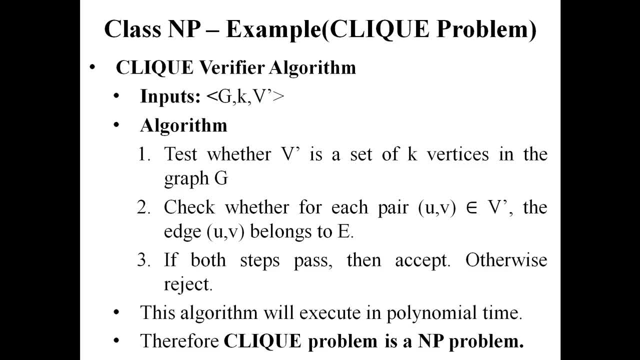 V dash is the subset of the vertex in the given graph. This verification algorithm checks if there is a click in the size of K between these V dashes. Since the size of the click is K, there should be K distinct vertices in V dash. 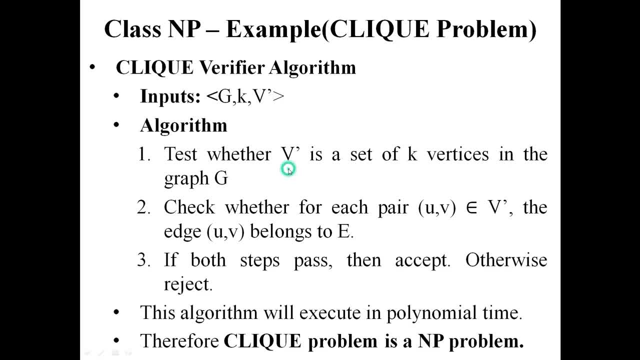 First of all we check if there are any. Then we take each pair of vertices in V dash. In between we check if there is an edge exist. All nodes exist only if there are edges in between. If both cases are successful, we can say that V dash is a click in the size of K in the graph G. 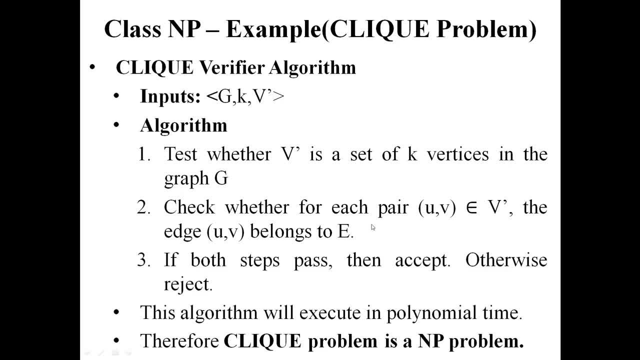 Or just reject it. Complexity of this algorithm is polynomial type. Click is a click in the size of K. To solve the click problem there is no polynomial type algorithm, but there is a polynomial type verifier algorithm. So click problem is a NV problem. 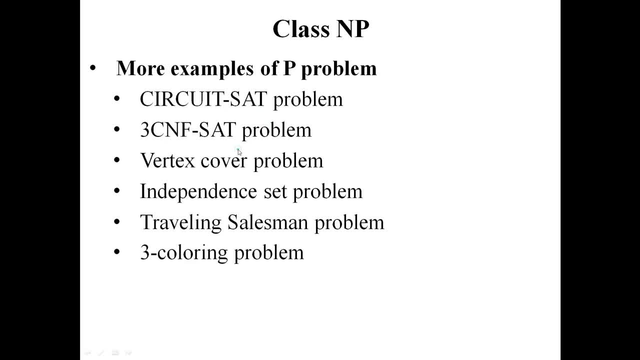 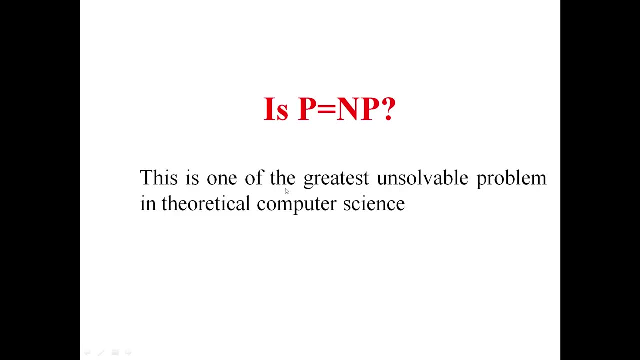 Some more examples: Circuit set problem, 3CNF set problem, vertex cover problem, independent set problem, travel in seismic problem, 3 coloring problem, etc. Is PE? This is one of the greatest unsolvable problem in theoretical computer science. 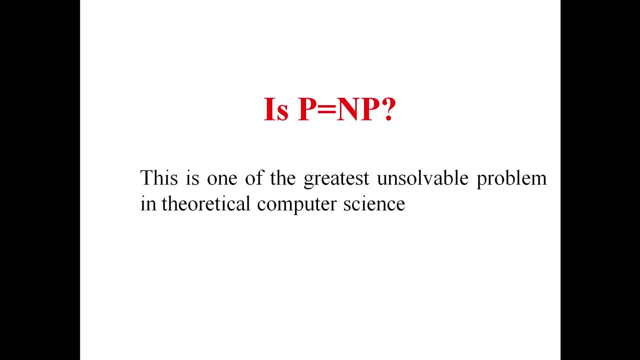 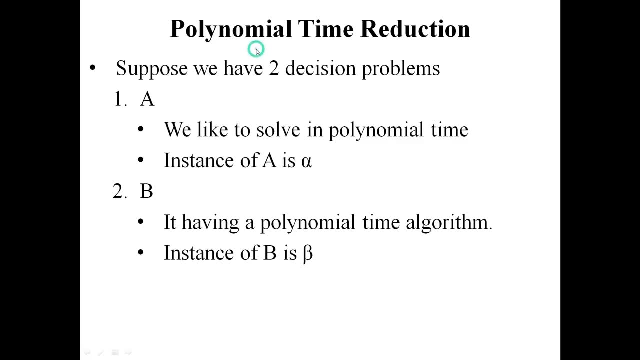 PE is not equal to NV. This is an open question. Next is polynomial time reduction. Suppose we have two decision problems. Decision problem means the output of that problem is either yes or no. No, it is not a. no, A and B are two decision problems. 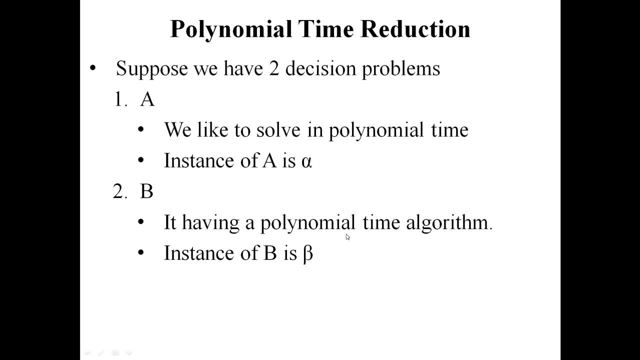 B already has a polynomial time algorithm, But A doesn't have such an algorithm. But we would like to solve the problem A in polynomial time. Instance of A is alpha. Remember, the input is the instance. Instance of A is alpha. Instance of B is negative. 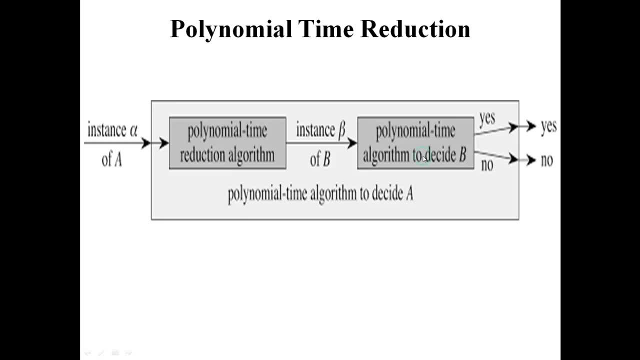 is beta. This is polynomial time decision. algorithm of B. The instance of A is alpha, The instance of B is beta. The algorithm of alpha to beta conversion is this algorithm reduction algorithm? Assume that this is happening in polynomial time For problem A at present. 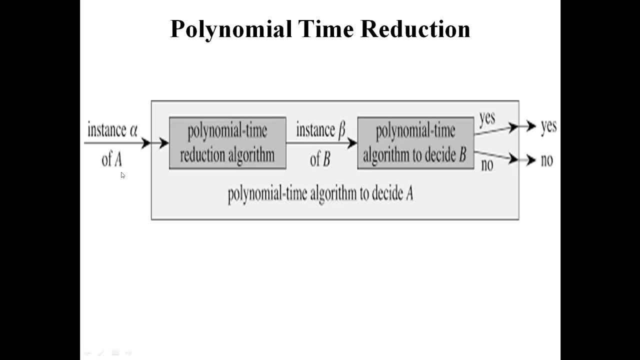 polynomial time algorithm is not existing. Assume that this is happening in polynomial time. Instead of executing A, A's instance, alpha is converted to beta and algorithm B is executed. If this is done, problem A can be solved in polynomial time. First part is reduction. This is in polynomial time. 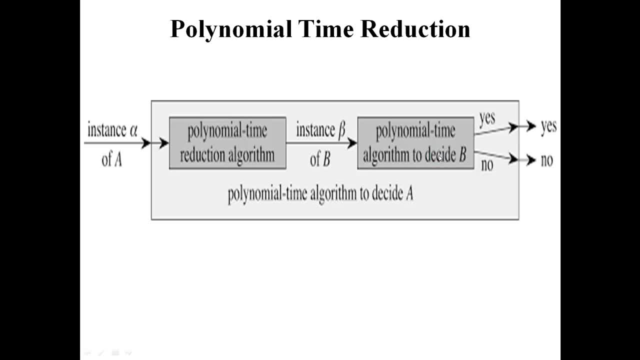 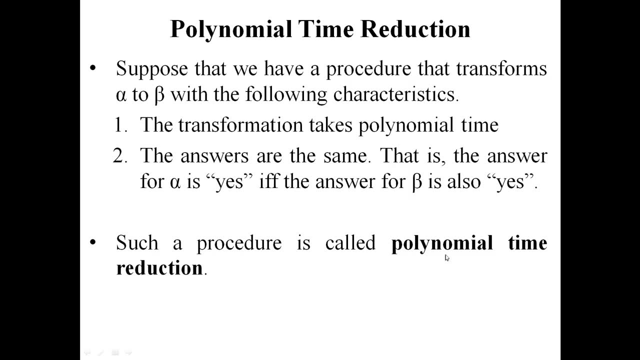 Then algorithm B is also in polynomial time. All right, All together. the complexity of solving problem A is polynomial. Polynomial time reduction algorithm should follow two properties. First thing: alpha to beta conversion should be in polynomial time. Second one: the answers are the same. 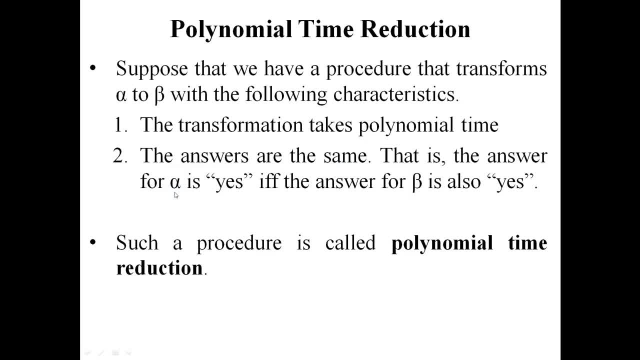 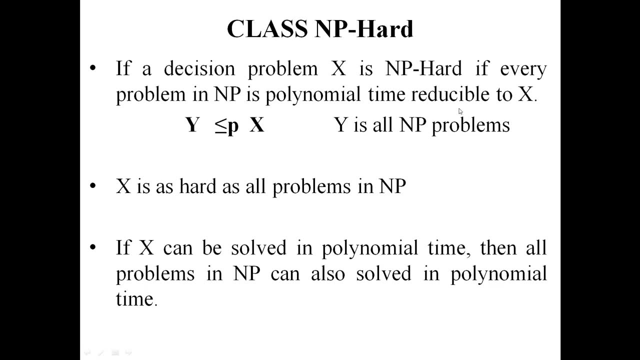 That means, if the answer is yes when problem A is executed with alpha, then the answer should be yes when B is executed with beta. The second property is polynomial time reduction algorithm. Third complexity class is NB-hard. Suppose X is a decision problem. 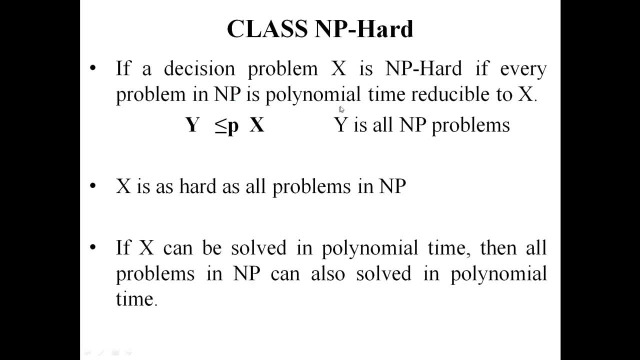 If all NB problems can be reduced to X in polynomial time, then X is called NB-hard. Y is polynomial time reducible to X. Y is all NB problems. X is as hard as all problems in NB If X can be solved in polynomial time. 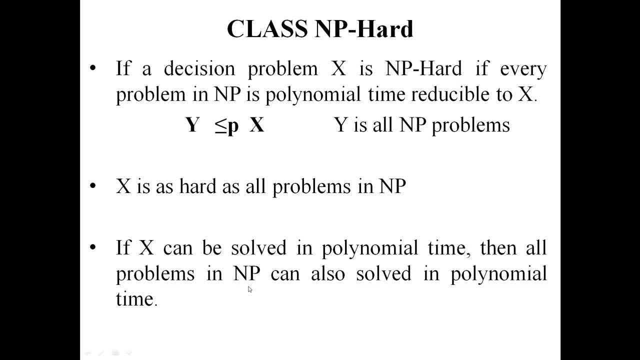 then all NB problems can be solved in polynomial time, Because all NB problems can be reduced to X in polynomial time. So any problem can be reduced to X in NB problem. Use the polynomial time algorithm of X and solve it. No algorithm has been found yet to solve any NB-hard problem in polynomial time. 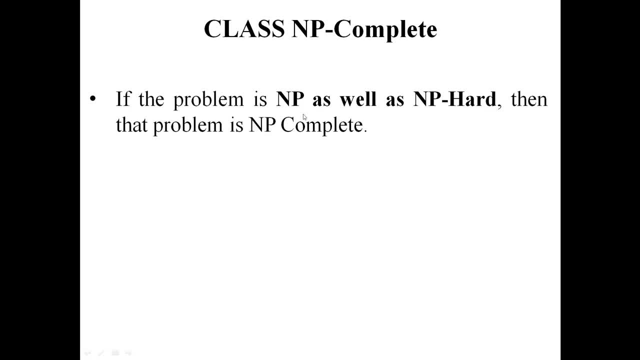 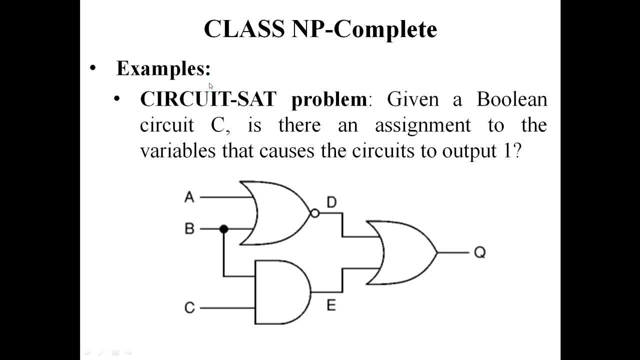 Next class is NB-complete. If a problem is both NB-hard and NB-hard then it is called NB-complete. Examples of NB-complete problems. First one is circuit set problem A Boolean circuit C will be given. Suppose this is the Boolean circuit. 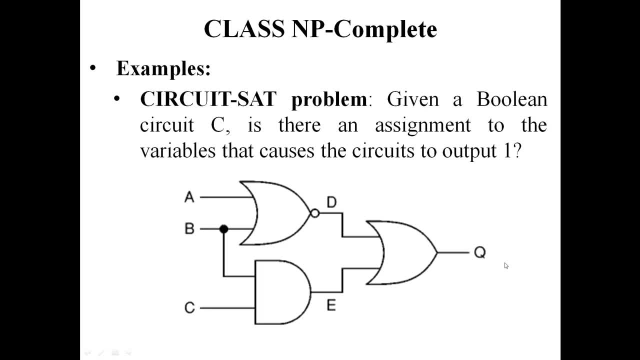 Its inputs are A, B, C. Output is Q In the direction of Q1,. A, B, C will have any possible assignments. Circuit set problem is a decision problem. Output is either Yes or No In the direction of Q1,. 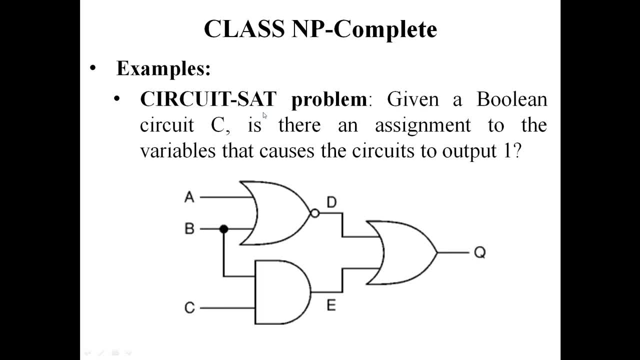 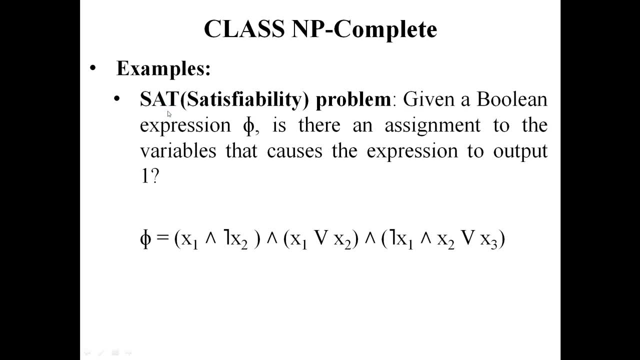 A, B, C will have any possible assignments. Circuit set result is Yes or No. Second example is SAT problem or Satisfiability problem. We will be given a Boolean expression: 5.. There are some variables in this. Here there are three variables: X1, X2, and X3. 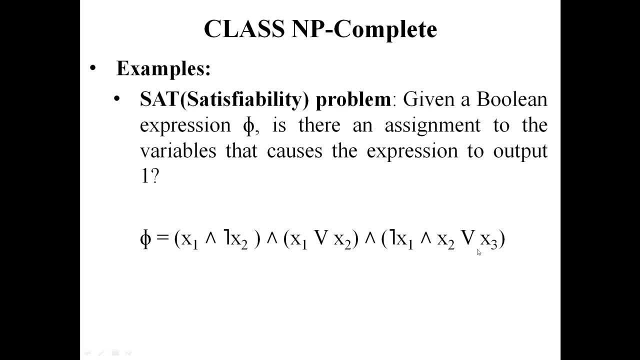 It is possible that its values are either 1 or 0. The variables are connected with AND and OR In any particular combination of these variables. is the result of the expression 1 or not? If it is 1, SAT problem will return Yes. 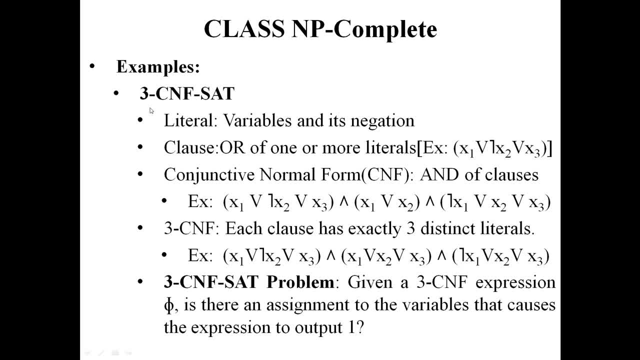 Otherwise it will return No. Third one is 3CN of SAT. Before saying what is 3CN of SAT, let us see some terms. First one is literal. Literal is the negation of a Boolean expression Clause. Clause is connected with OR. 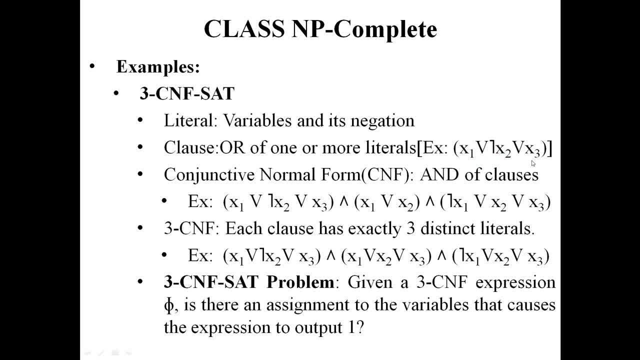 Here X1, negation, X2, X3 are the three literals It is connected with OR, So this one is called a clause. Next is Conjunctive Normal Form, or CNF. CNF is connected with AND of clauses. 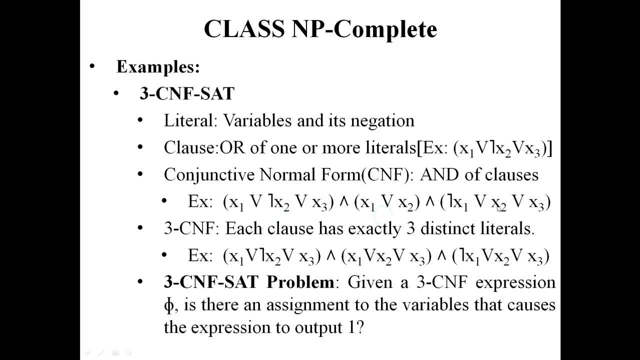 Here we have three clauses. This is first one, second one, third one. There is an AND operator in between each clause, So the entire expression is in CNF. Next is 3CNF If there are exactly three distinct literals in each clause. 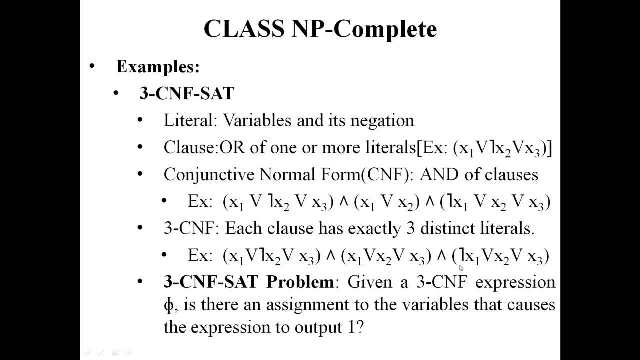 it is called 3CNF. This is an expression in 3CNF. In each clause three distinct literals are placed, So it is in 3CNF. Next, what is 3CNF SAT problem If there is a 3CNF expression. 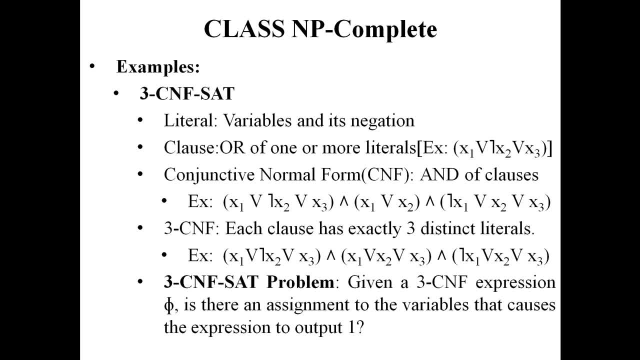 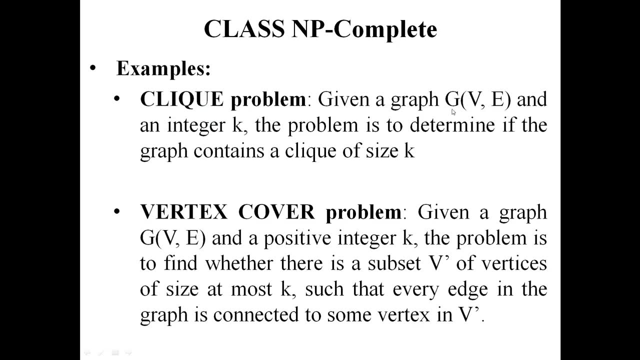 is there an output 1 in any possible assignments of the variables? If there is 1, 3CNF, SAT will return YES, Otherwise NO. Next example is CLICK problem. Is there a CLICK in the case size of the given graph G? 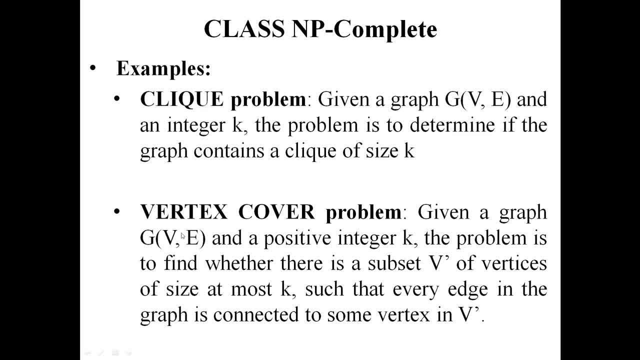 Is the output of this also YES or NO? Next example is Vertex Cover Problem. A. graph G is given. Its vertices are V. The subset of V is V' Assume that the size of V' is K, Is it possible to cover all the edges of the graph using these K nodes? 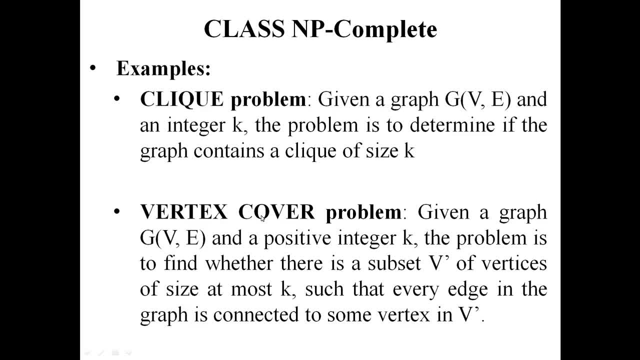 The answer to this is either YES or NO.